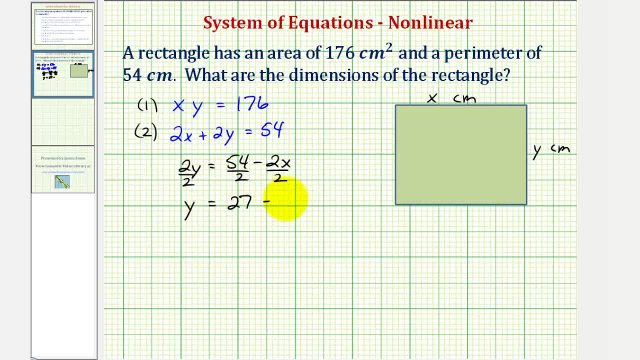 So we know that y must equal 27 minus x, And since y is equal to 27 minus x, we can replace y with 27 minus x- 27 minus x- in this first equation- and then solve for x. So by substitution we would have the equation. 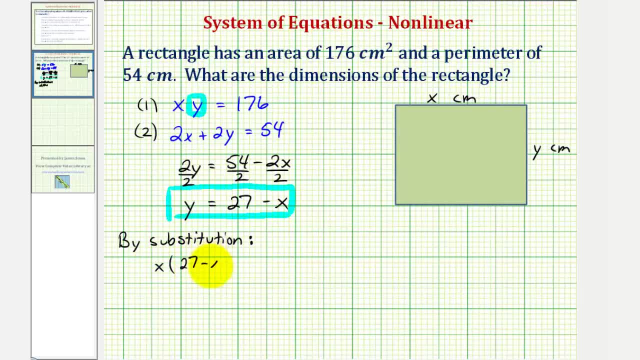 x times the quantity 27 minus x must equal 176.. Now we'll put the parentheses by distributing x. That would give us 27x minus x squared equals 176.. Notice, we have a quadratic equation. so we'll set this equal to zero and solve for x. 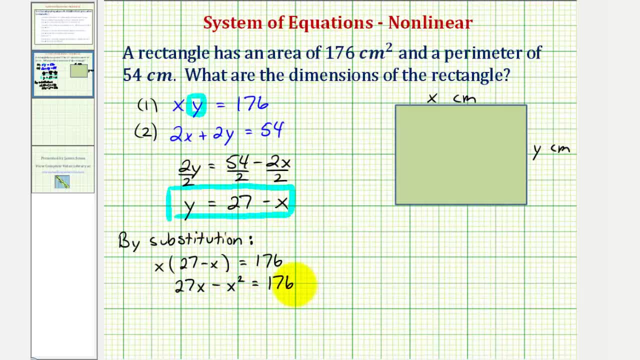 We prefer to have the x squared term positive, so let's go ahead and add x squared to both sides, as well as subtract 27x on both sides. That would give us the equation: zero equals x squared minus 27x plus 176.. 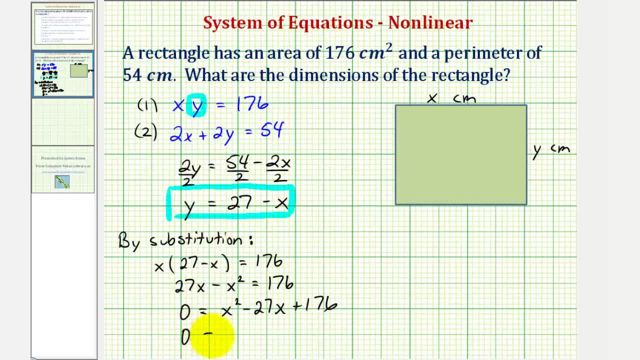 Now, if this does factor, it'll factor into two binomial factors, where the first positions must come from the factors of x squared, So x squared, which are x and x. The second terms would be the factors of 176 that add to negative 27.. 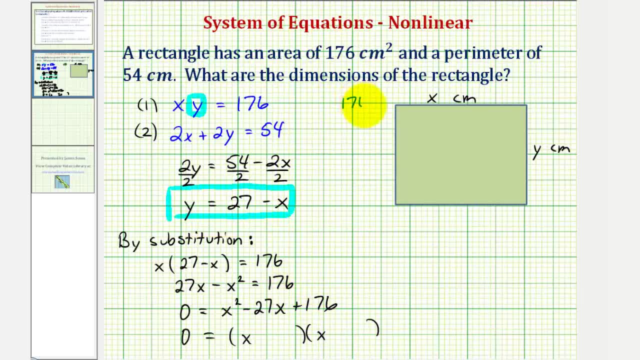 That's not an easy question. but if we start to break down 176 into its prime factors, we could start with two times 88.. We could break down 88 into eight times 11.. And notice, if we stop here, this shows us that 16 times 11 is equal to 176,. 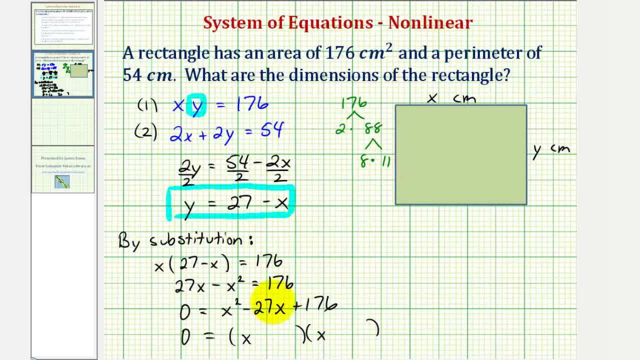 and 16 plus 11, is equal to 27.. And since we want negative 27,, we could use a factor of negative 16 and a factor of negative 11,, which would give us a product of 176 and would sum to negative 27.. 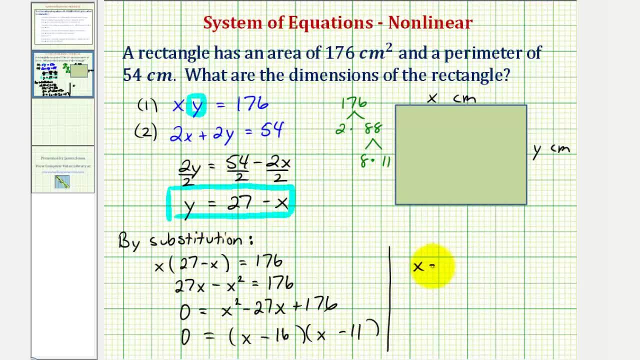 So notice how we have two solutions to this equation. We have x equals positive 16, or x equals positive 11.. It may seem strange to have two possible values for x, but notice how, if x is 16,, y is equal to 27 minus 16, or 11..